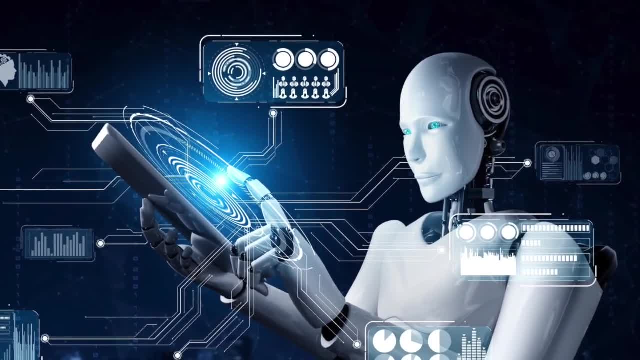 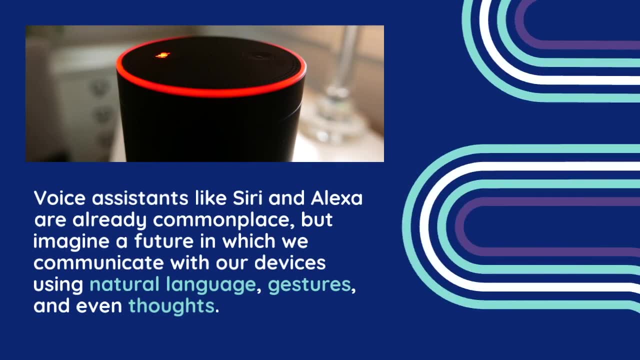 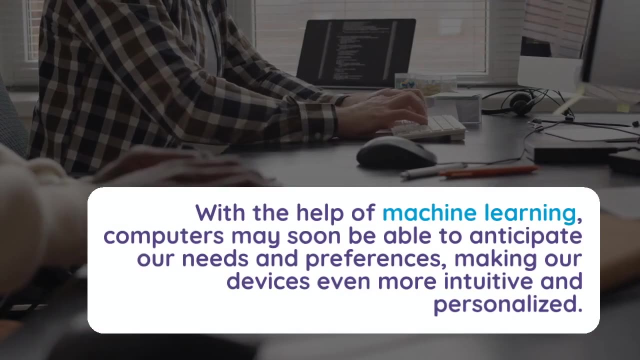 and machine learning are making it possible for computers to better understand and respond to human input. Voice assistants like Siri and Alexa are already commonplace, But imagine a future in which we communicate with our devices using natural language, gestures and even thoughts. With the help of machine learning, computers may soon be able to understand and understand. 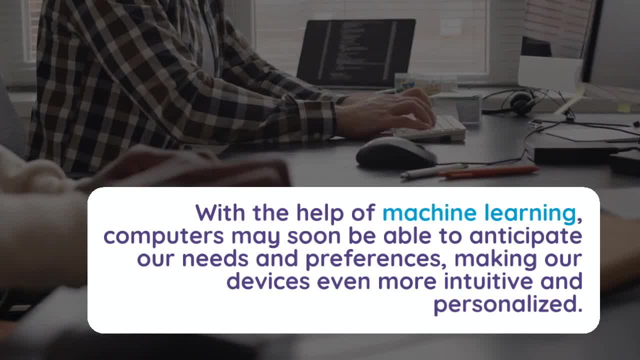 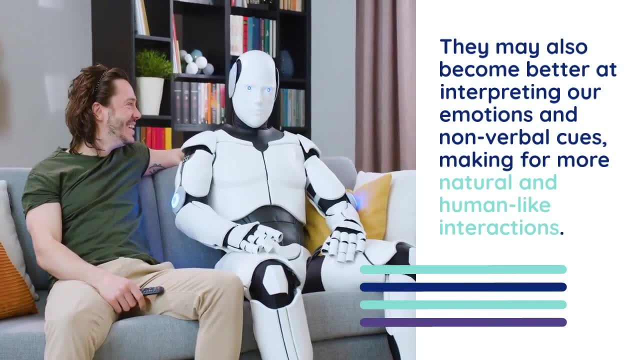 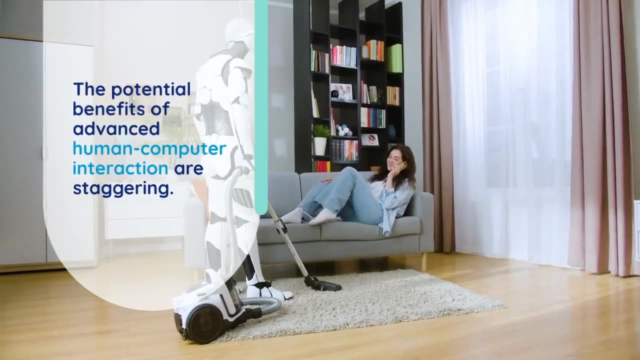 our needs and preferences, making our devices even more intuitive and personalized. They may also become better at interpreting our emotions and non-verbal cues, making for more natural and human-like interactions. The potential benefits of advanced human-computer interaction are staggering: By making it easier to access, 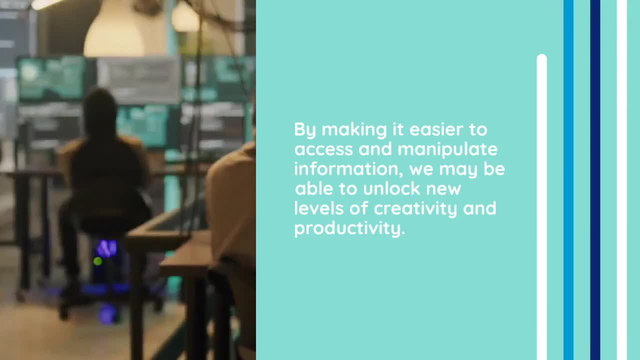 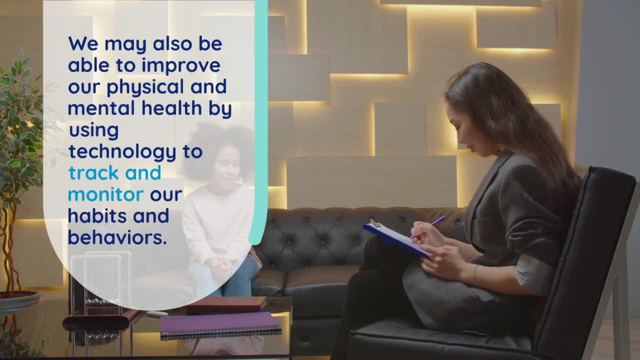 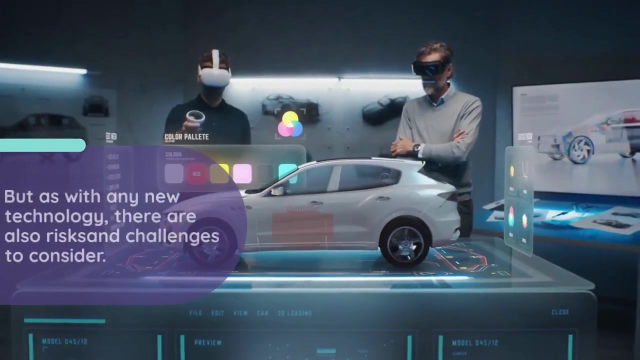 and manipulate information, we may be able to unlock new levels of creativity and productivity. We may also be able to improve our physical and mental health by using technology to track and monitor our habits and behaviors. 3. The challenges of human-computer interaction and AR. But as with any new technology, there 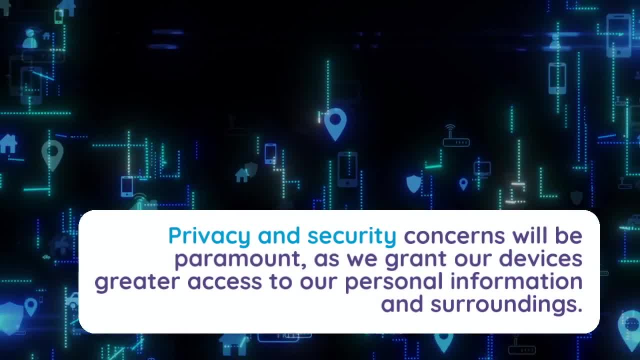 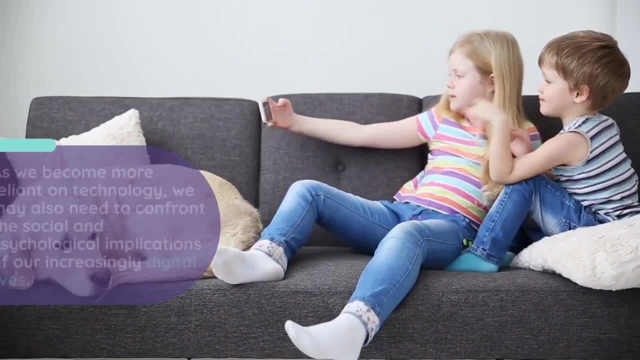 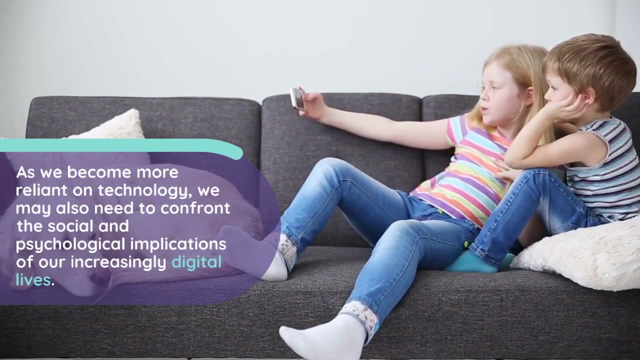 are also risks and challenges to consider. Privacy and security concerns will be paramount as we grant our devices greater access to our personal information and surroundings. As we become more reliant on technology, we may also need to confront the social and psychological implications of our increasingly digital lives. For example, we may need to grapple with the 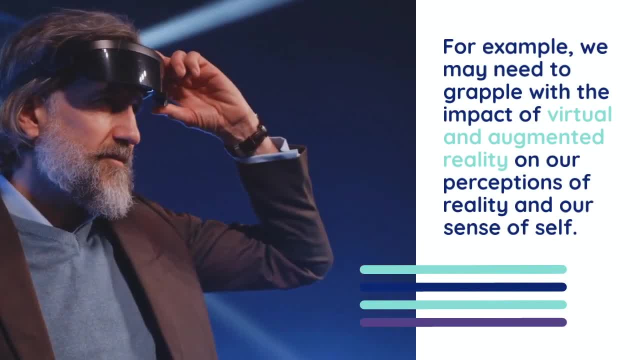 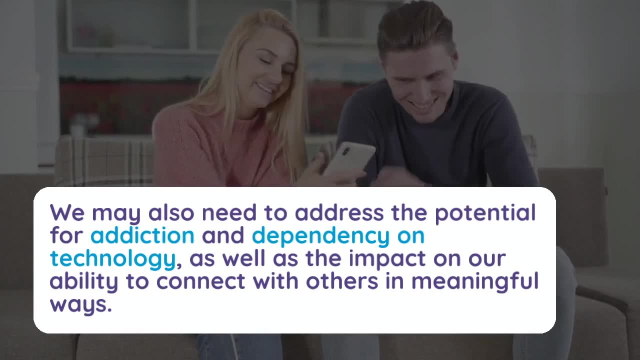 impact of digital technology on our lives. We may also need to confront the social and psychological implications of virtual and augmented reality on our perceptions of reality and our sense of self. We may also need to address the potential for addiction and dependency on technology, as well as the impact on our ability to connect with others in meaningful